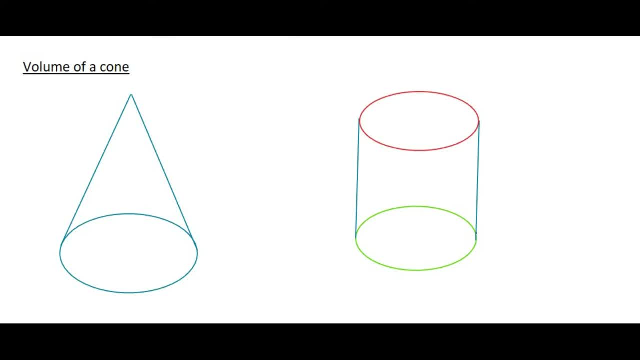 In this video we will be looking at the volume of a cone, But first can you remember what the formula is for volume? Well, volume is equal to the area of the base times the height. And so if we were looking at a cylinder, which we have here on the right, 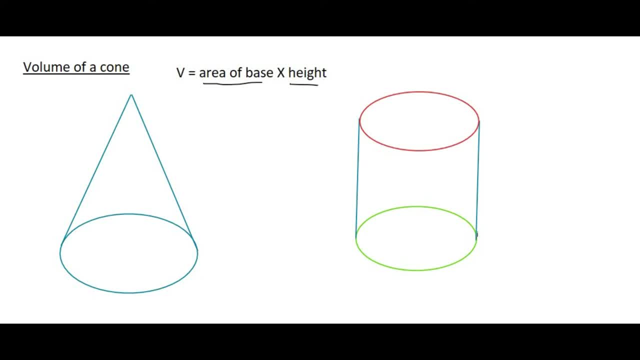 then we could use the base, for example, as the circle at the bottom, And then what we would do is we would drag that circle up to the very top and that length would be the height, And so the final. for that cylinder. we would say: volume is equal to, so the area of the base would be a circle. 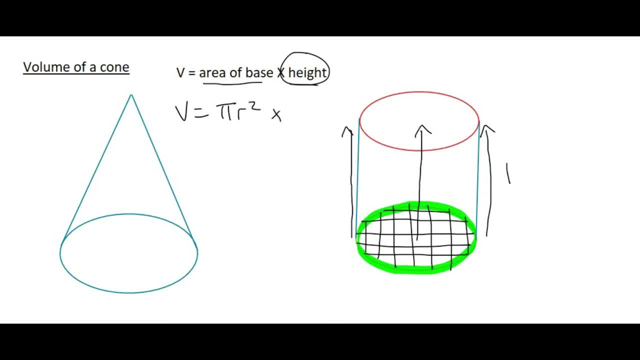 so that would be pi r squared, And then the height we would use would be this height over here. So you would do something like that. But that's a cylinder. In this video we're talking about a cone, but they do have a similarity. Would you say that you could put more water in the cylinder? 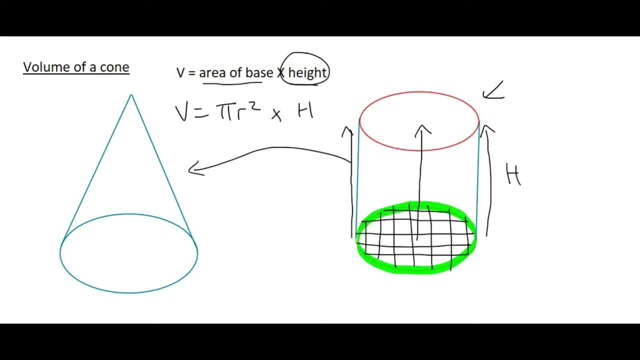 or could you put more water in the cone? if their radius and their height is the same, Well, it's obvious that you would be able to fit more water in the cylinder, Because all of this part over here has been taken away. when you're looking at a cone, 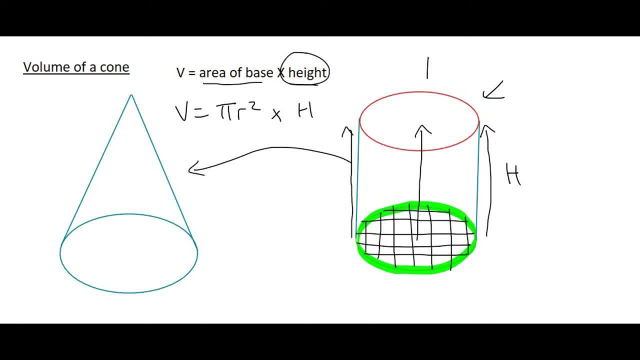 And so mathematicians have come up with a rule that we can use whenever we have a pyramid kind of shape. Now, a pyramid kind of shape is anything where it starts off wide at the bottom and then ends up narrow or at a specific point at the top. 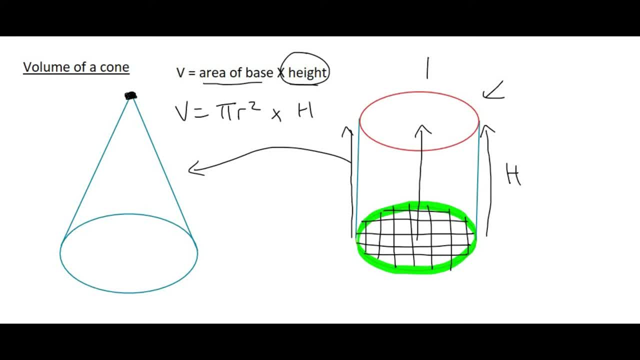 So what mathematicians- and you might remember this from when we did the cube and the pyramid- we said that all you have to do at the end is divide your answer by three. So what you could do is you could imagine this cylinder over here. you would get that one's answer. 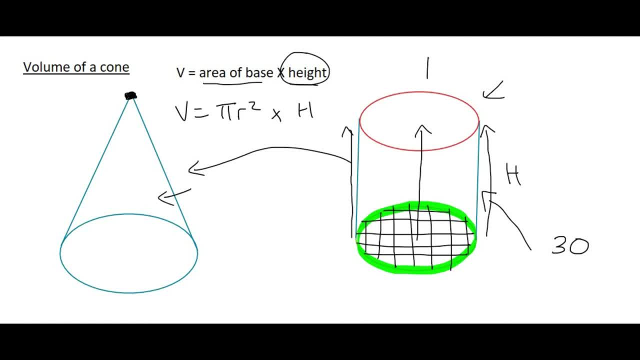 And let's say the volume was 30. Then for the cylinder you would just say 30 divided by three, And so the volume of a cone is equal to the following: So there it is. at the bottom It says the area of base times height. So you do that and that would be the same as for a cylinder. 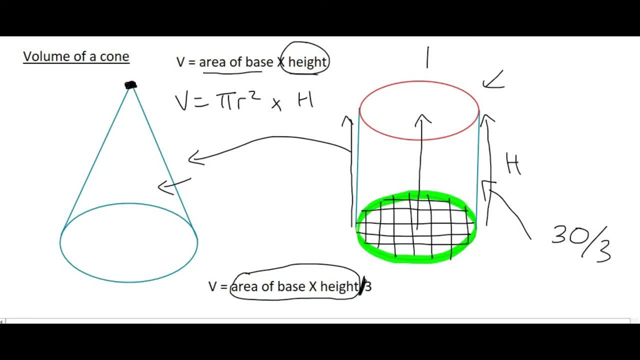 And then that little line is me trying to say: divide. So you then say: divide it by three. And so in your in class your teacher might use the following. She might say: or he or she might say: volume is equal to a third a times H.